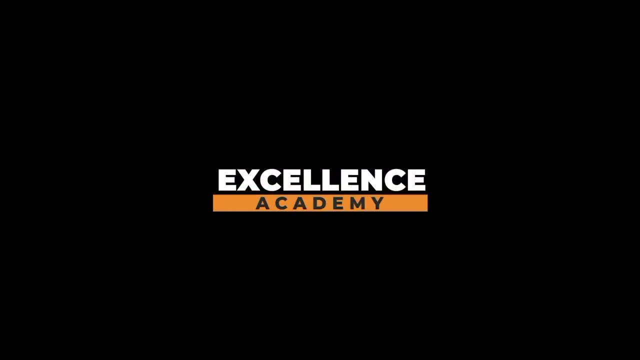 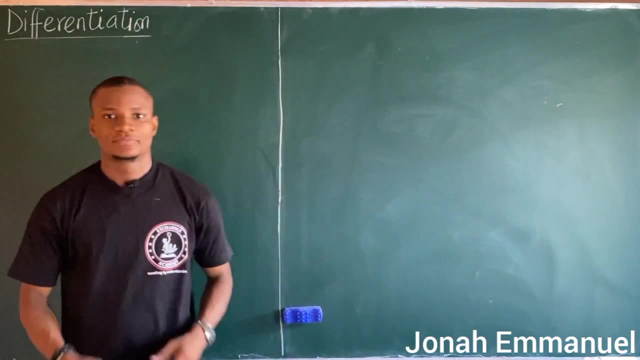 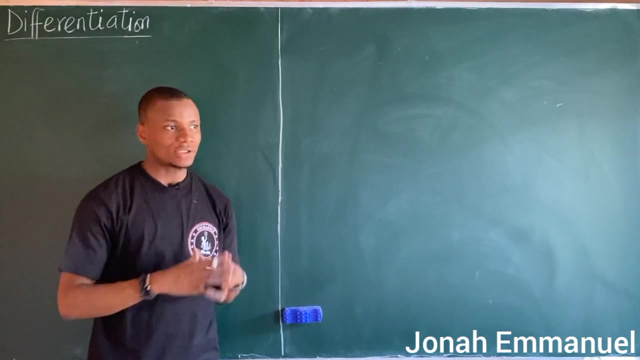 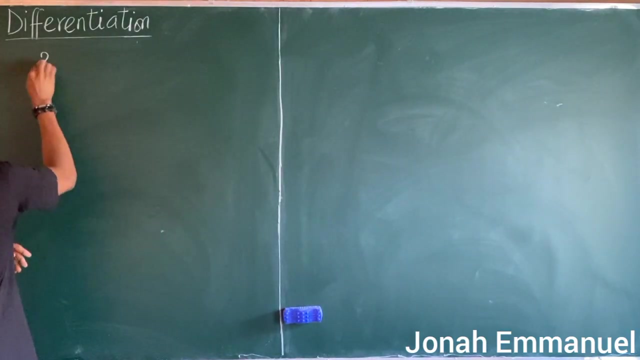 hello and welcome to excellence Academy. today we'll be looking at the third method of differentiation, and that's chain rule. all right, so method three for differentiation, and that's chain rule. all right, so here's your hint. chain rule is used when I have a number of 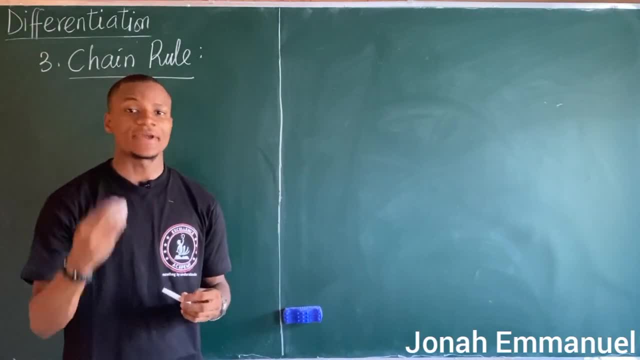 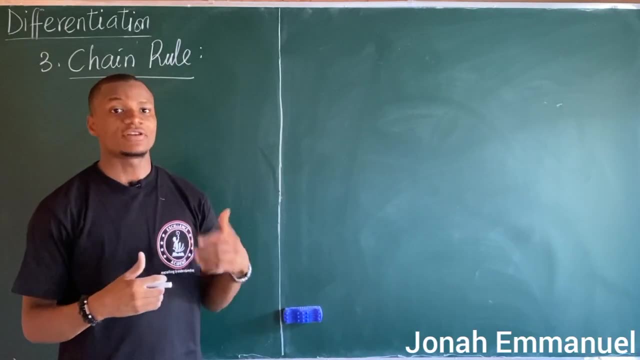 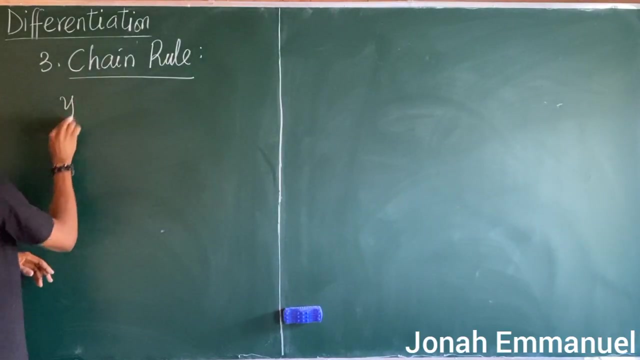 things: either adding or subtracting being raised to a path. right, what I have a number of times: either adding themselves or subtracting being raised to a certain path, or perhaps complex paths. for instance, if I have that Y is equal to- let me take 6 plus X- 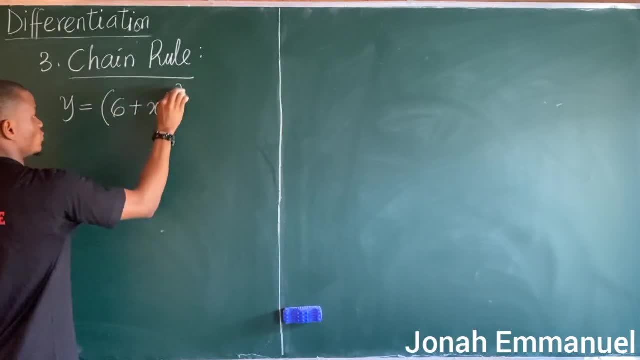 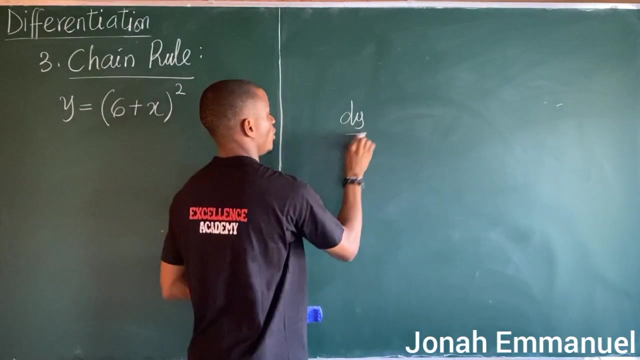 for instance, or the path 2: right, so for this case here I will use chain rule. the other methods you could use here will consider this one much more later. all right, so with this case 1, what the concept behind chain rule? for chain rule, I have that dy all over dx is equal to dy all over. 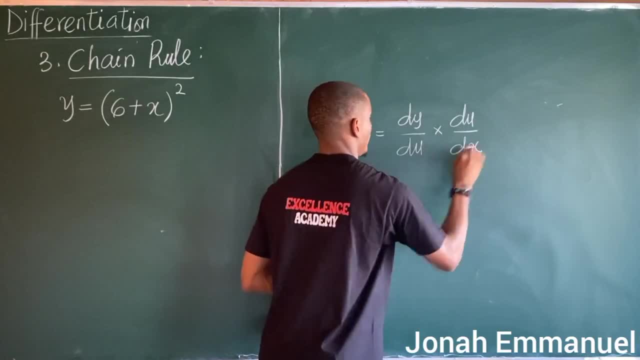 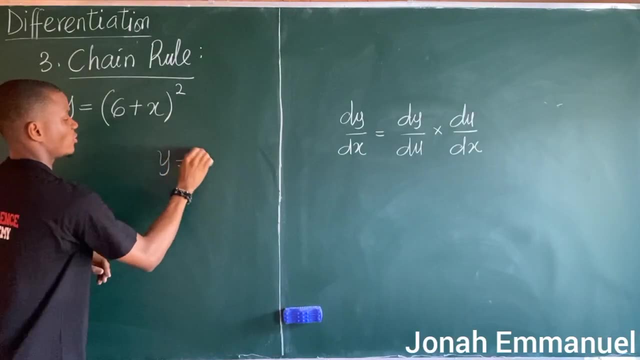 the X. all right. so here's your case. what if I had Y being equal to X? square from this now, obviously you know that the one by the X is equal to what here? 2x, using general method. so for this now, what if I have Y being equal to 6 plus X, or the path 2? what about the X? 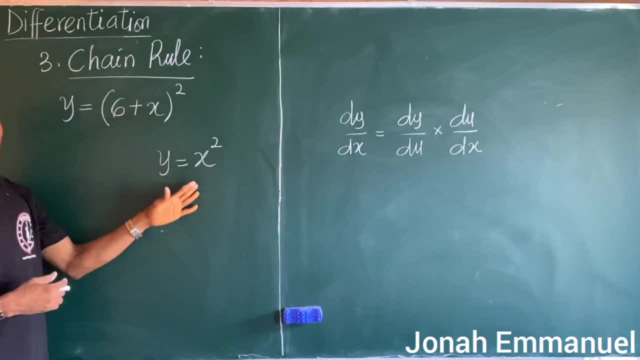 here. it's not as easy as this right now. why is that so? if you observe, the paths are the same. so why this is so is because in this case now i now have a much more complex um case as compared to this. this was a single number or a single term to part two. this is now um double 10 to part two. 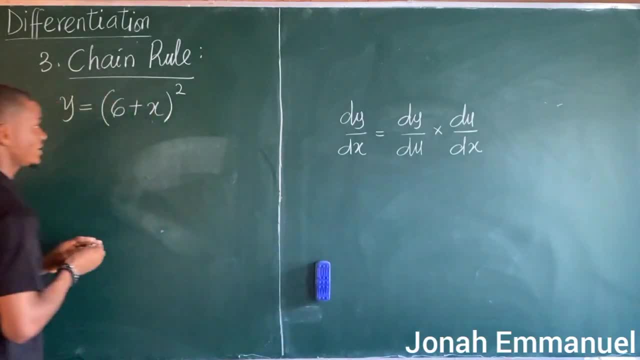 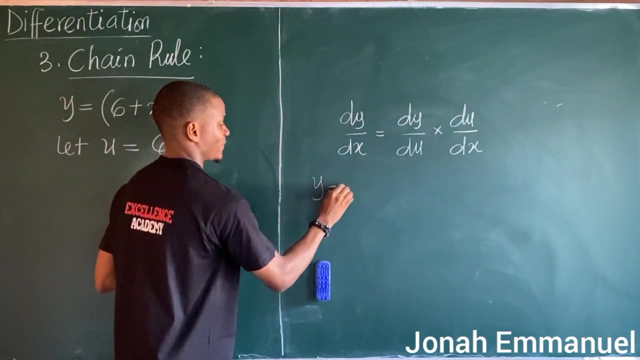 so the case will now be this: for this, now the case will be: i will say: let u be equal to what i have in my brackets. so use one term to represent everything in the brackets. so u is equal to what there: 6 plus x, all right next up, um, when i had y expressed in terms of x, we said: if i differentiate, 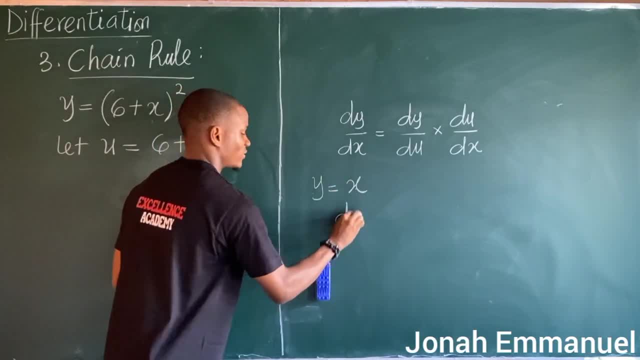 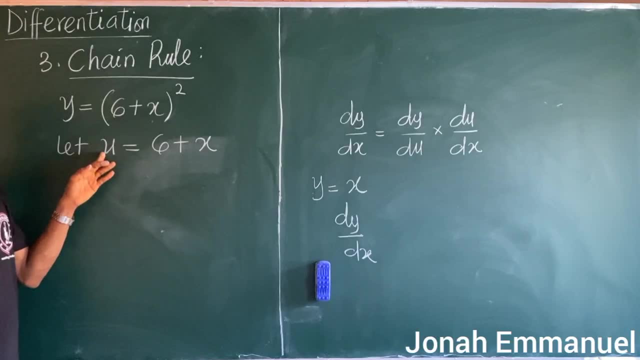 y with respect to x, it gives you what? there the y all over the x. but this is not the case here. in this case, now, i have u expressed in terms of x, so if i differentiate this, it gives you what? now the u over the x, please. 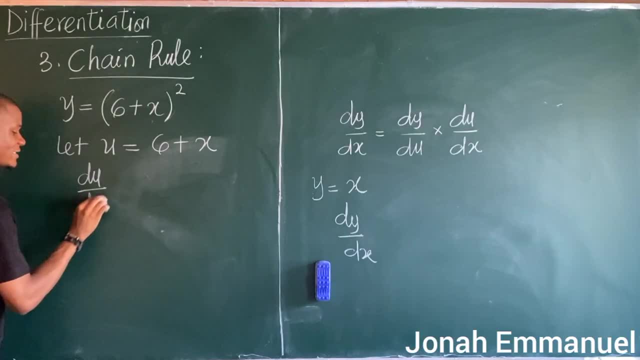 so it becomes the u all over, the x is equal to. for this now, obviously i'll use my general method. if i differentiate six, a constant gives you what there zero, so i'm having zero. plus differentiate x gives you what there one, so i'm having one which equal to one, so i have that. 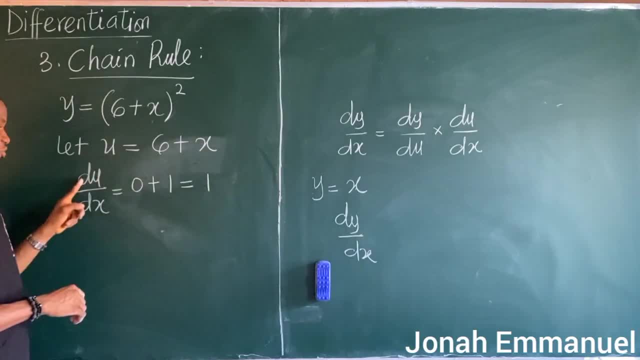 if u is equal to six plus x, the u over the x. on differentiating this, i'll have one next up. i have that y is now equal to um. why was this? but we said all of this should be equal to what you, so i'm using you to represent all of this. so y is now equal to this is. 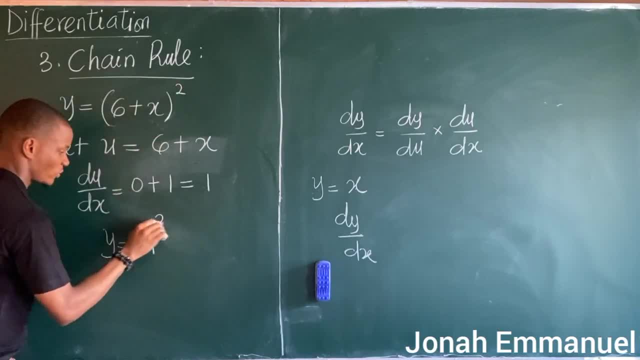 u, it becomes u 1. here u squared. if i differentiate y with respect to u now gives you what there, please dy over du. observe, i differentiated you with respect to x. it gave me du over dx. i am now to differentiate y with respect to u. it gives you what there dy over du. so i'll have that dy over du. is now equal to y over u and that's y over x and d y over d x. divided times: y with respect to y. we can see now. lets us start now. give us in brother u. so i've differentiated y with respect to u by uorge i התjährล清楚. 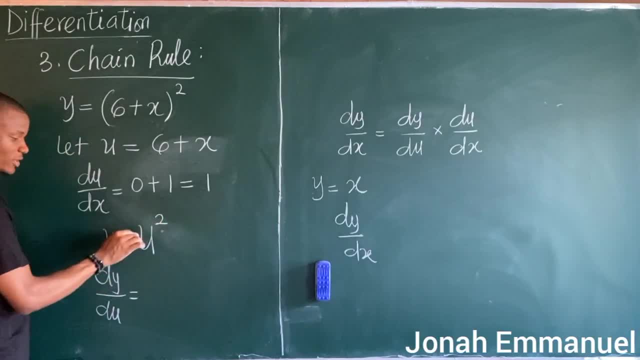 quartzo, absolutely so. if i do that, i'm differentiating y mildly. plus in theophysis i now get that. so the whose difference? but it's up to you. so now, is it not that i want that there, the fish. i'll use general method here. so this gives you here. i'm having two u into two minus one is one.